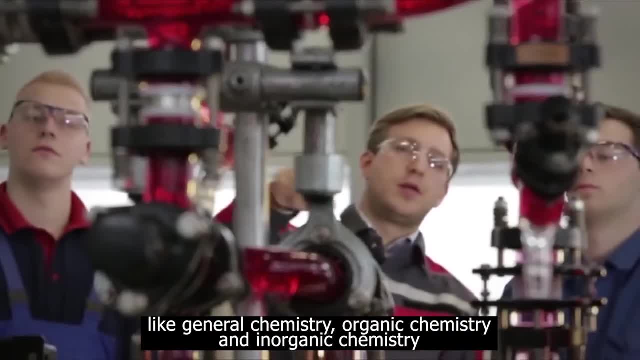 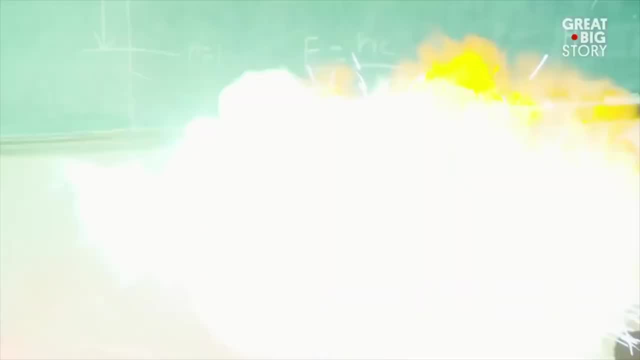 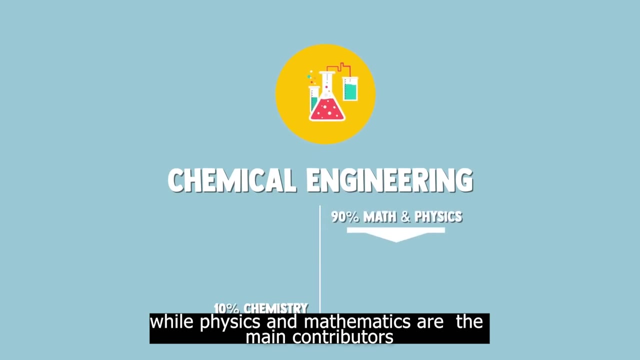 chemistry, organic chemistry and inorganic chemistry, as well as the physics behind the reactions, such as thermodynamics and fluid dynamics. In fact, chemistry only plays a small part in chemical engineering, while physics and mathematics are the main contributors. With such knowledge, a chemical engineering graduate should be able to do a lot of research. 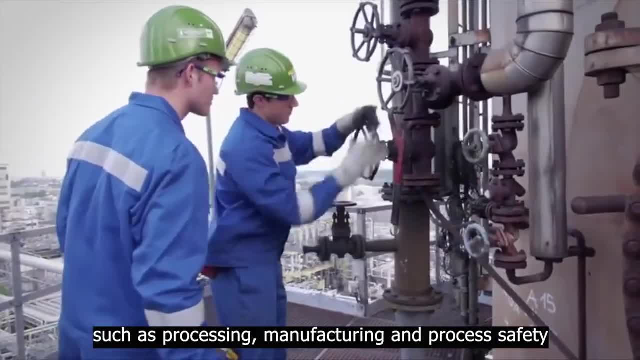 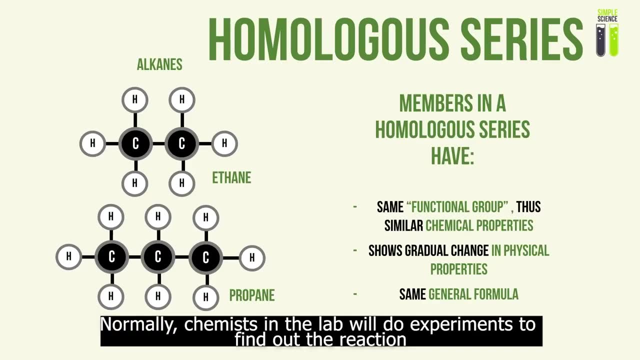 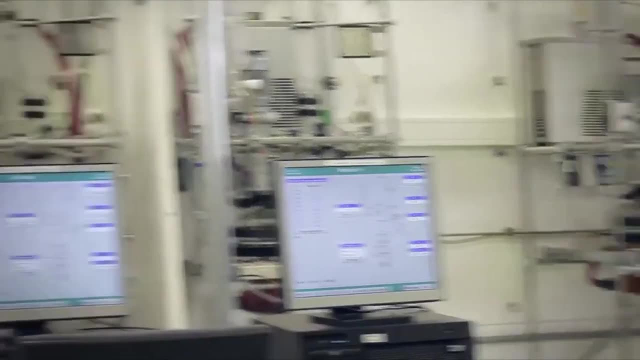 and can decide various paths in the industry, such as processing, manufacturing and process safety. Normally chemists in the lab will do experiments to find out the reaction to produce the desired product. Meanwhile, chemical engineers will take the experiment, the process and the procedure to produce it on a larger scale. 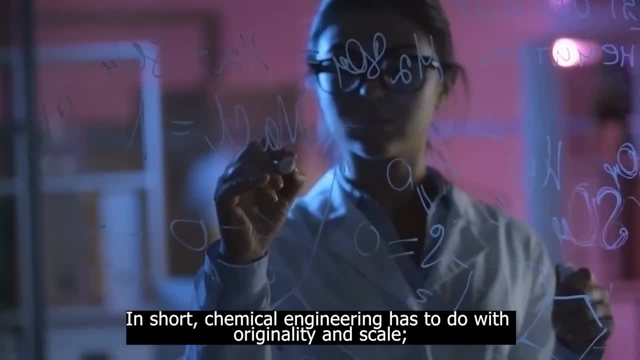 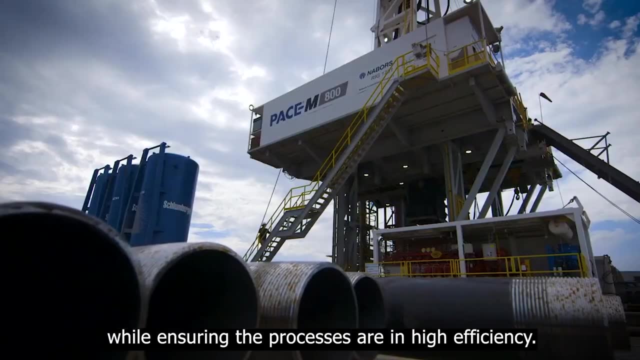 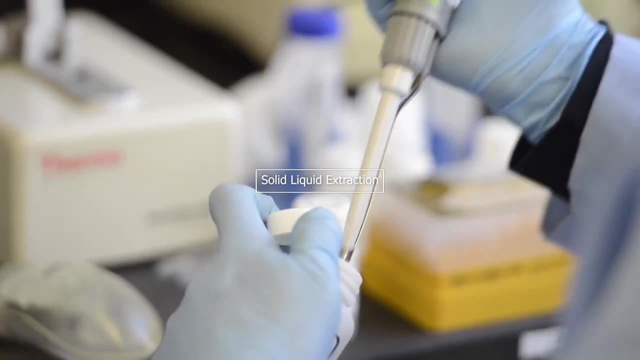 In short, chemical engineering has to do with originality and scale. They use the materials and process them to produce the product. In the process, chemical engineers will take them to an industrial scale while ensuring the processes are in high efficiency. After getting to know what chemical engineering is all about, let's talk about solid-liquid. 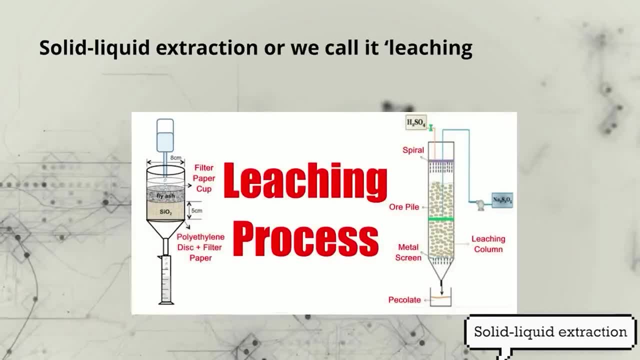 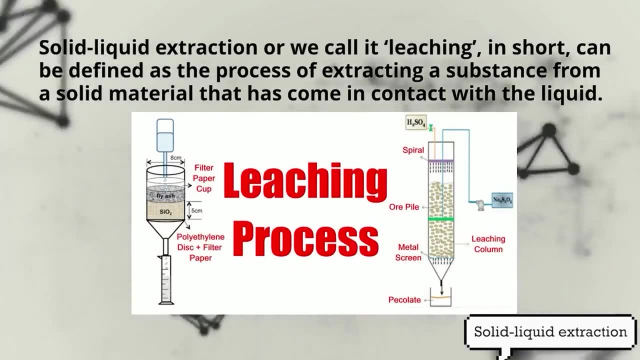 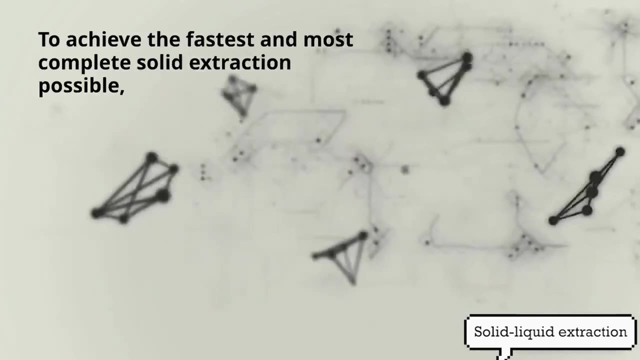 extraction. Solid-liquid extraction, or we call it as leaching in short, can be defined as the process of extracting a substance from a solid material that has come into contact with the liquid To achieve the fastest and most complete solid extraction possible. we 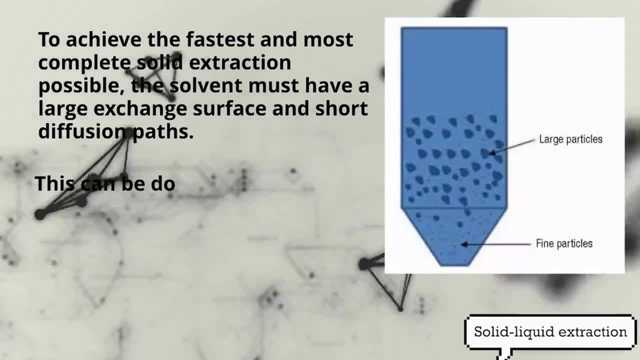 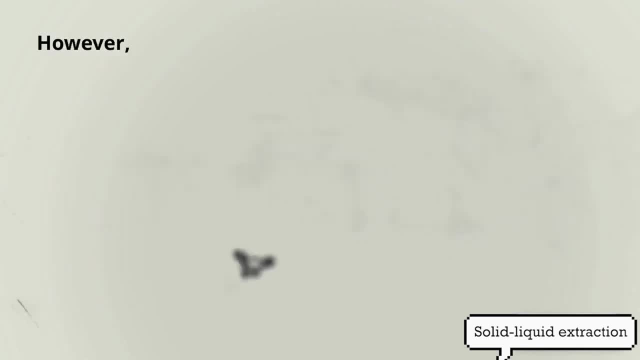 need to know the structure of the liquid. The solution must have a large exchange surface and short diffusion path. This can be done by reducing the solid to be extracted into very fine particles. However, we need to take note of the process, because an excessively 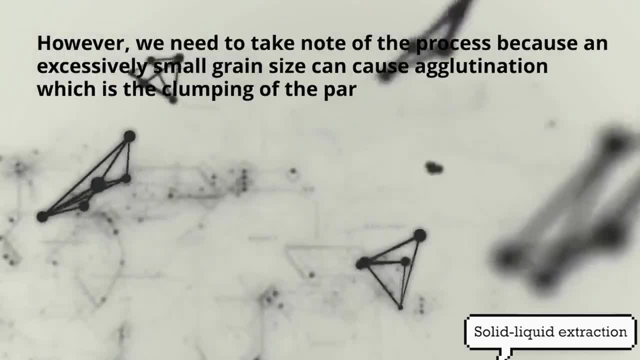 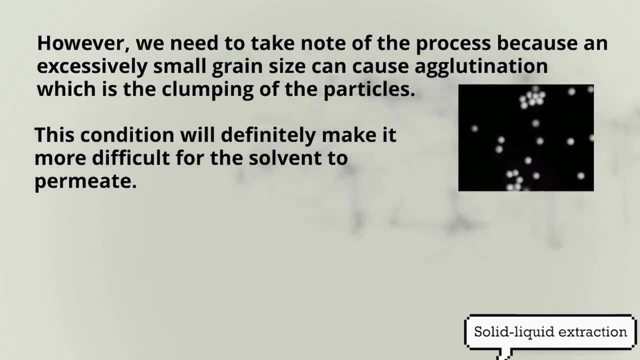 small grain size can cause agglutination, which is the clumping of the particles. This condition will definitely make it more difficult for the solvent to permeate. The simplest form of this unit operation is that the extraction must be done in a very high-density solution. The solution must be done in a very high-density solution. The solution must have a large exchange surface and short diffusion path. This can be done by reducing the solid to be extracted into very fine particles. The solution must be done in a very high-density solution, However. 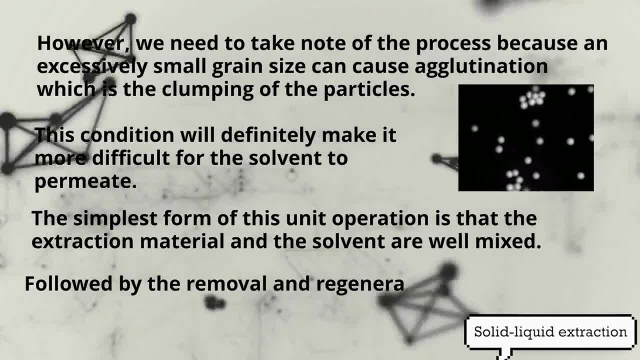 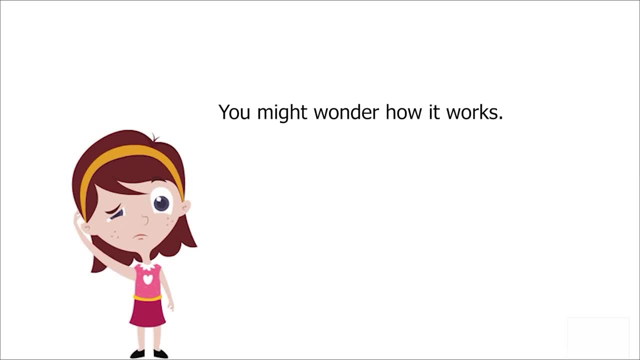 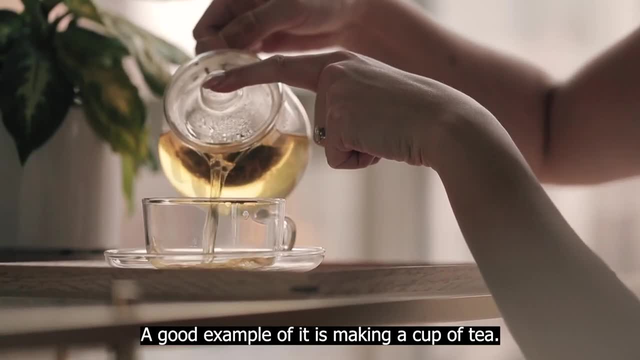 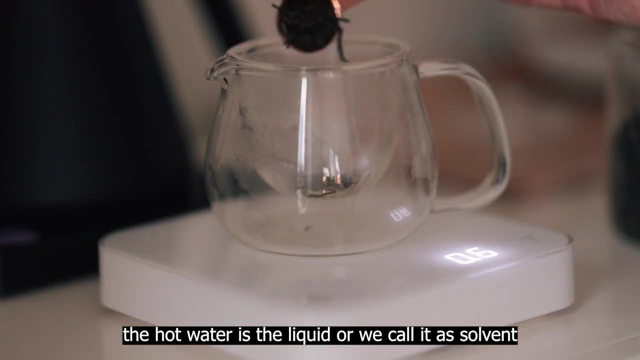 the extraction material and the solvent are well mixed, followed by the removal and regeneration of the solvent and the dissolved transition component. Solid-liquid extraction is actually practiced in our daily life as well. A good example of it is making a cup of tea. In this case, the tea leaves act as the solid, the hot water. 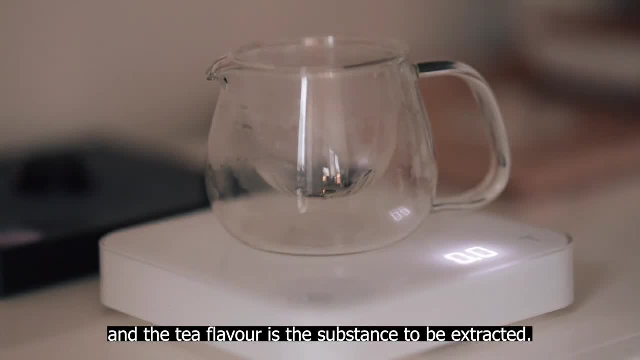 is the liquid or we call it as solvent. In this case, the tea leaves act as the solvent and the tea flavor is going to be the liquid. Solid-liquid extraction can be done. either flavor is a substance to be extracted. The soluble particles, which is the tea flavor, dissolve in the 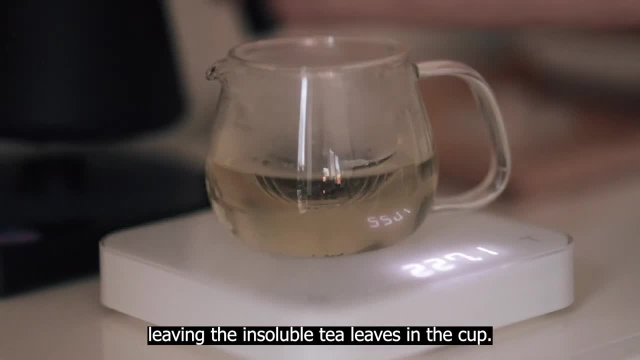 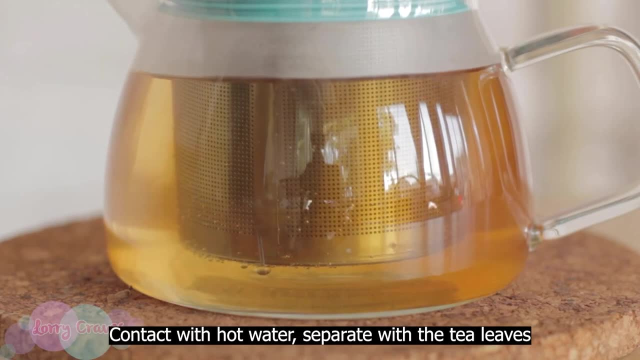 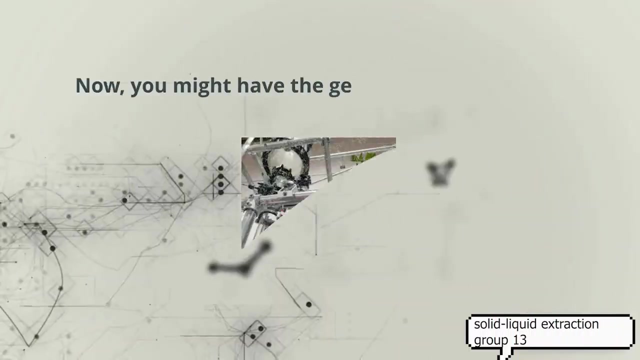 hot water, leaving the insoluble tea leaves in the cup. or it can be simplified as a process of contact, separate and extract: Contact with hot water, separate with the tea leaves and we extract the tea flavors. Now you might have the general idea of solid liquid extraction, So we will go. 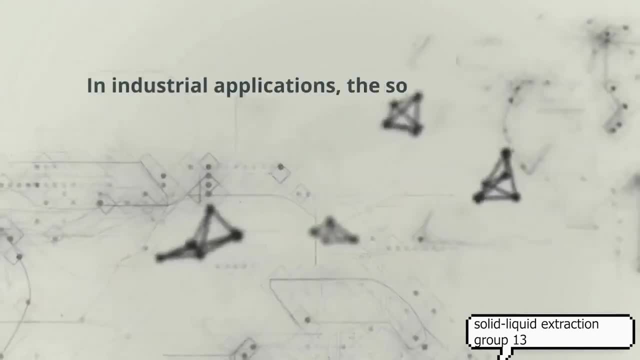 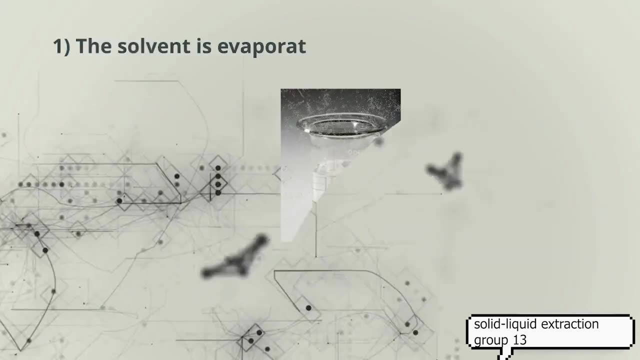 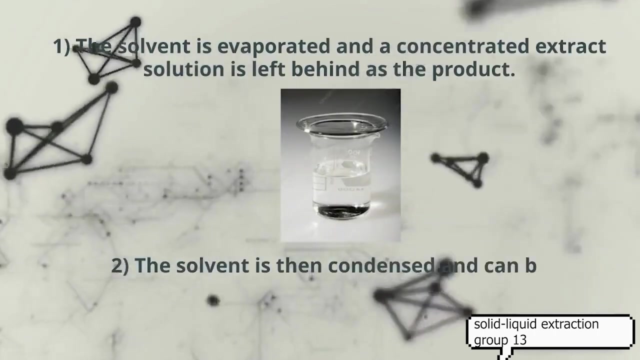 into industrial examples. In industrial applications, the solvent is normally regenerated using evaporation or distillation method. The solvent is evaporated and a concentrated extract solution is left behind as the product. The solvent is then condensed and can be reused. Before we go into details, let's take a look at what are the factors that will affect the 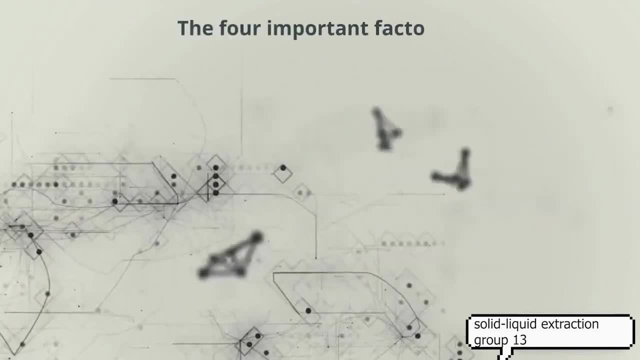 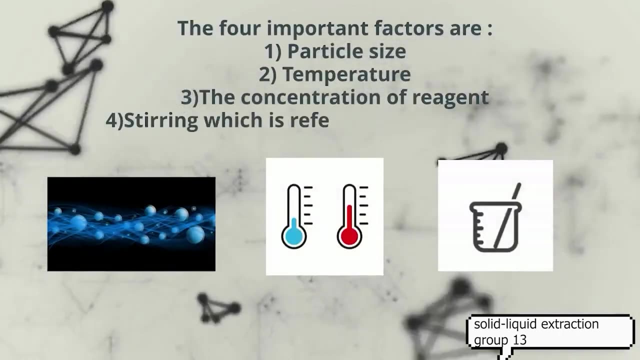 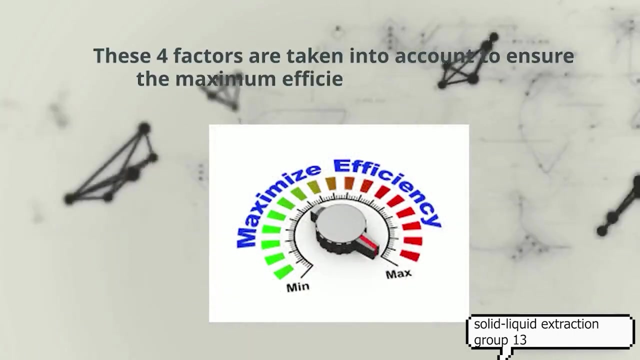 extraction rate. in the leaching process, The four important factors are: Particle Size, Temperature, Concentration of reagent and stirring, which is referring to the agitation of the fluid. These four factors are taken into account to ensure the maximum efficiency of the leaching outcome. 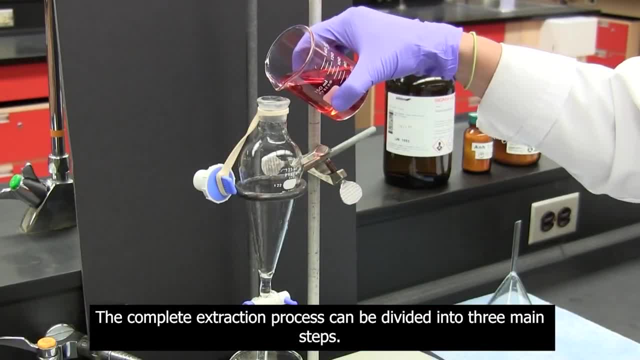 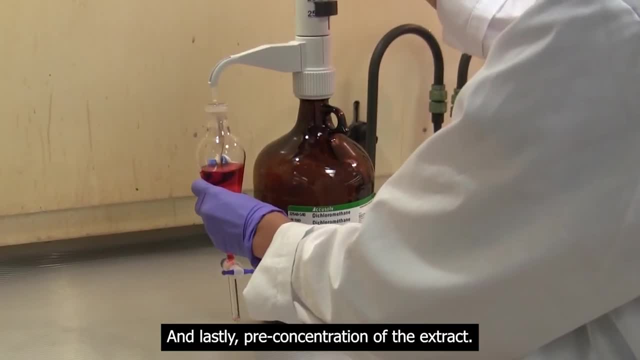 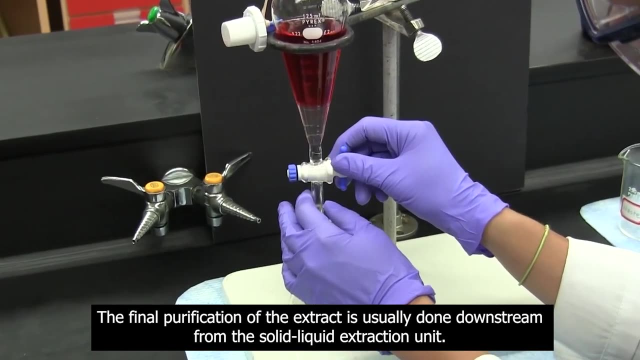 The complete extraction process can be divided into three main steps: First, preparation of solvent. Second, extraction process And lastly, pre-concentration of the extract. The final purification of the extract is usually done downstream from the solid liquid extraction unit. 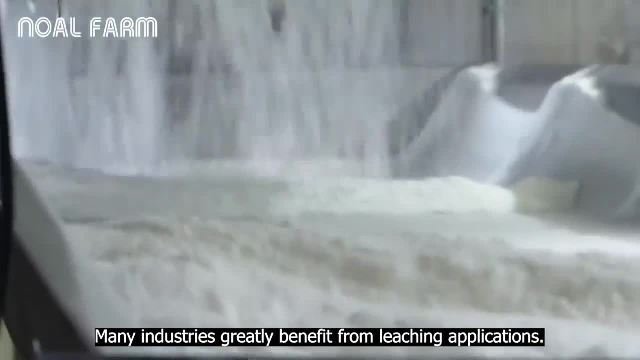 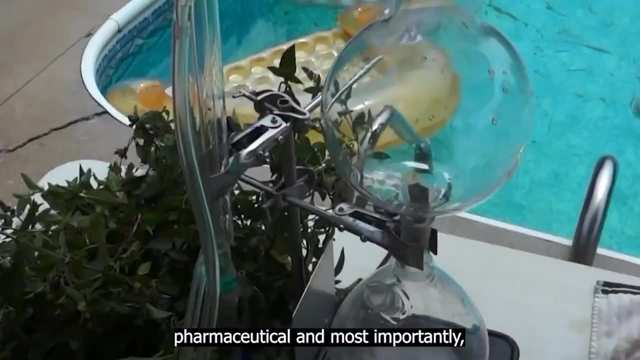 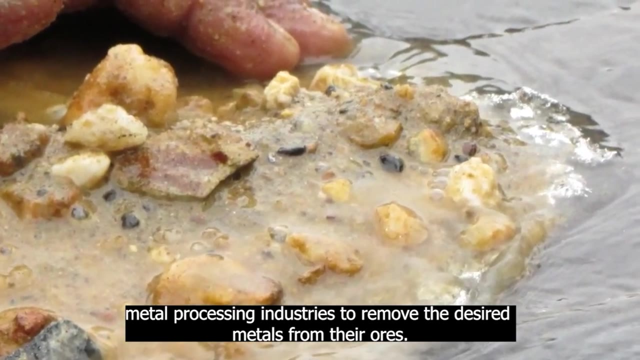 Leaching is actually widely used. Many industries greatly benefit from leaching applications, For example, biological and food processing industries, pharmaceutical and, most importantly, metal processing industries, to remove the desired metals from their ores. Examples for leaching in food industries are the separation of sugar. 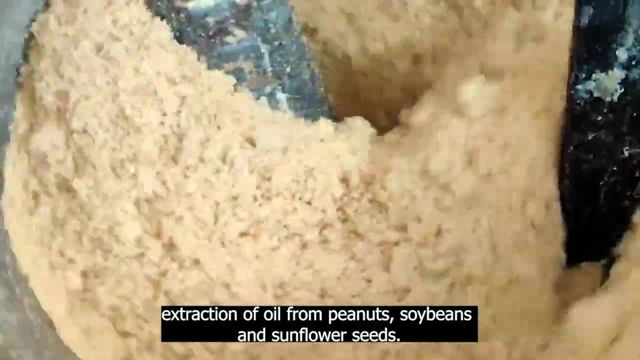 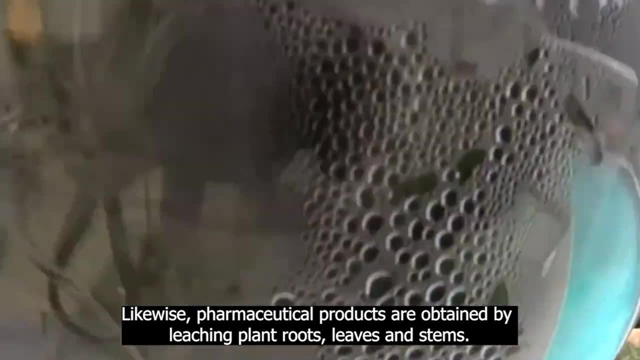 from sugar bits with hot water. The separation of sugar from sugar bits with hot water. The separation of sugar from sugar bits with hot water. Extraction of oil from peanuts, soybeans and sunflower seeds. Likewise, permac будете critical products are obtained by leaching plant roots, leaves and stems. 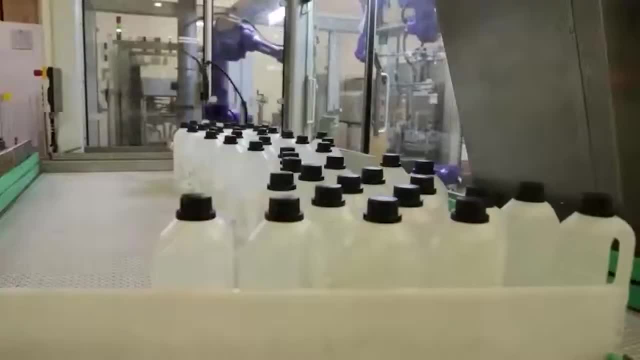 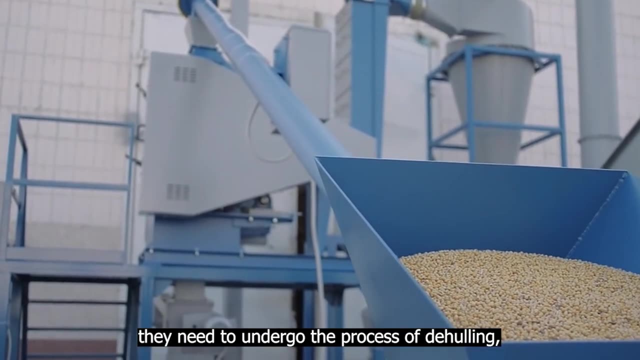 Now they will look detailed into some applications. Firstly, extraction of vegetable oil from soybeans. Before the soybeans are extracted, they need to undergo the process of dehealing, cleaning, cracking and flacking. Breastaing is the process of the skin avoiding O putting too much oil into the 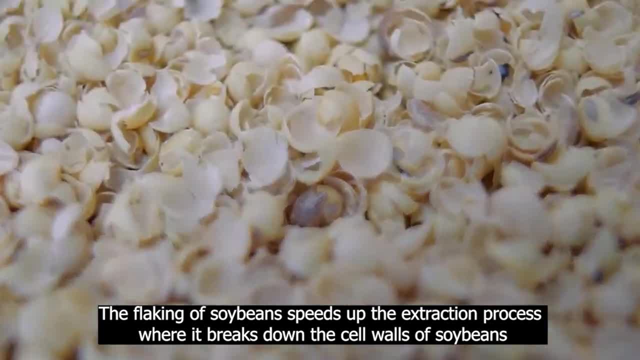 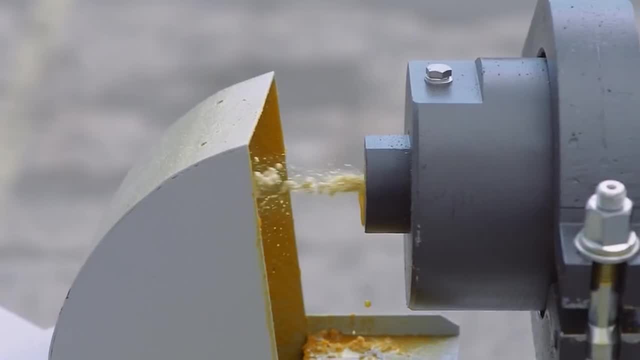 The flaking of soybeans speeds up the extraction process, where it breaks down the cell walls of soybeans, which allows the solvent to come into direct contact with the oil. For an ideal leaching of soybeans, the soybeans need to have a high oil solubility to minimize 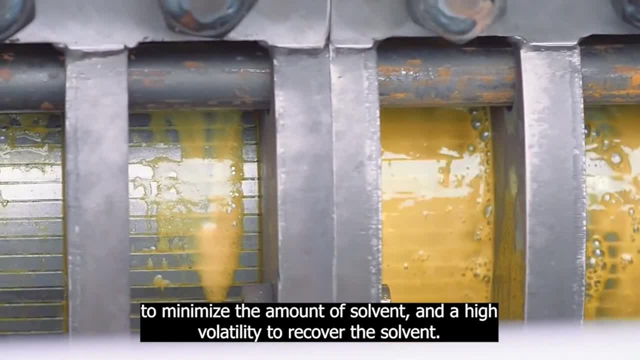 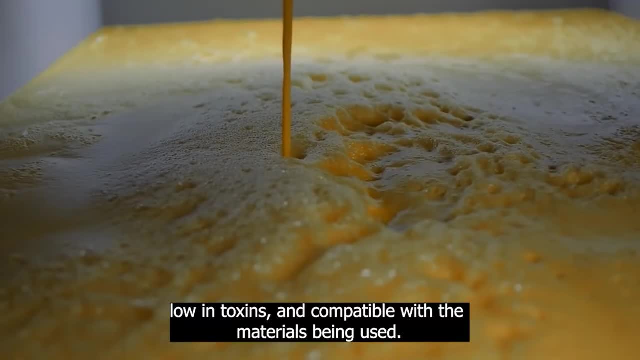 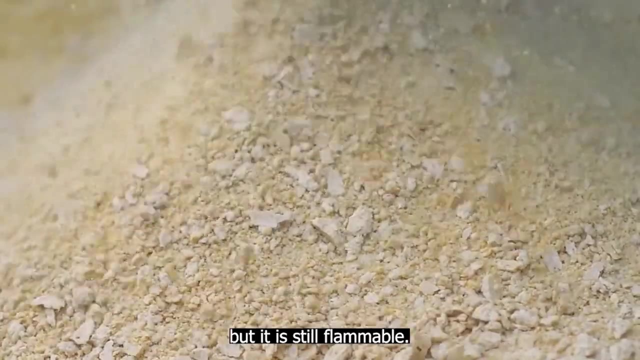 the amount of solvent and a high volatility. to recover the solvent, The soybeans also need to be non-flammable, low in toxins and compatible with the materials being used. Therefore, N-hexane is normally used, as it has a low toxicity, but it is still flammable. 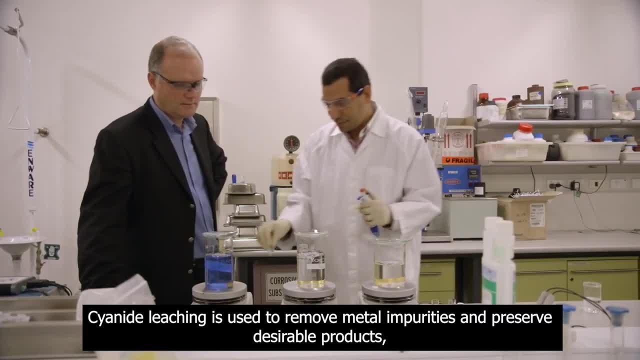 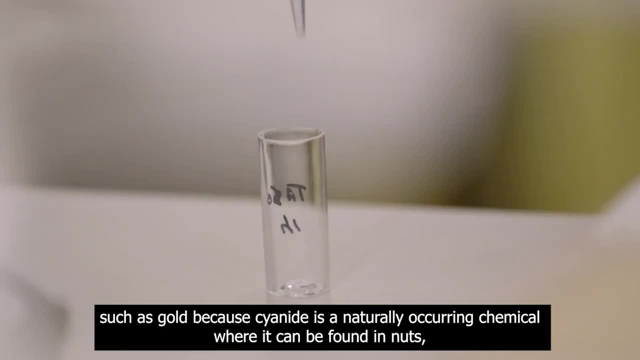 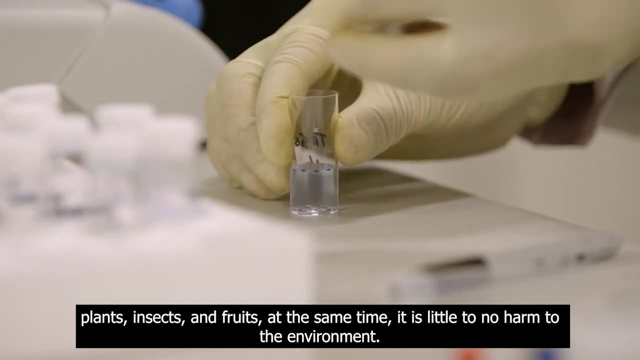 Next we look into gold leaching. Cyanide leaching is used to remove metal impurities and preserve desirable products such as gold, because cyanide is a naturally occurring chemical where it can be found in nuts, plants, insects and fruits. At the same time, it is lethal to no harm to the environment. 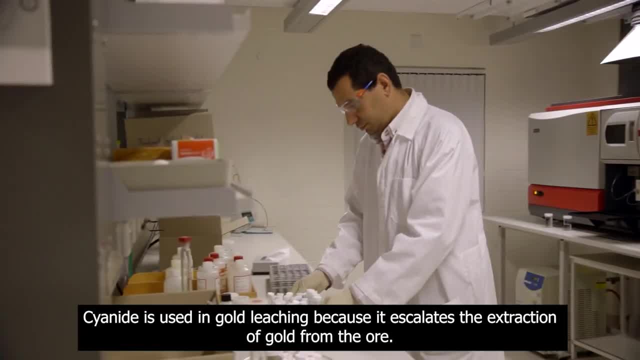 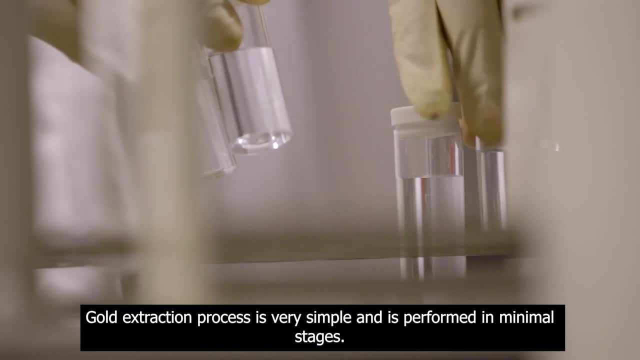 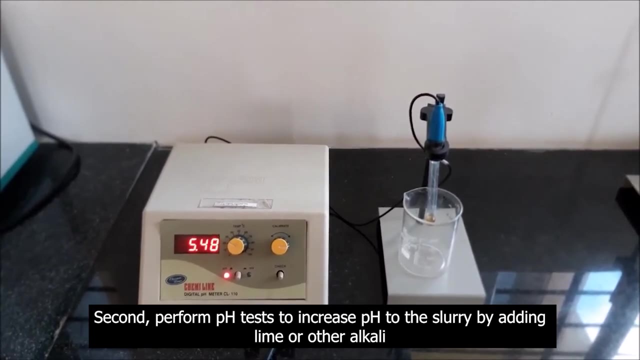 Cyanide is used in gold leaching because it escalates the extraction of gold from the ore. Gold extraction process is very simple and is performed in minimal stages: First, crush the ore. Second, perform pH test to increase pH to the slurry by adding lime or other alkaline. 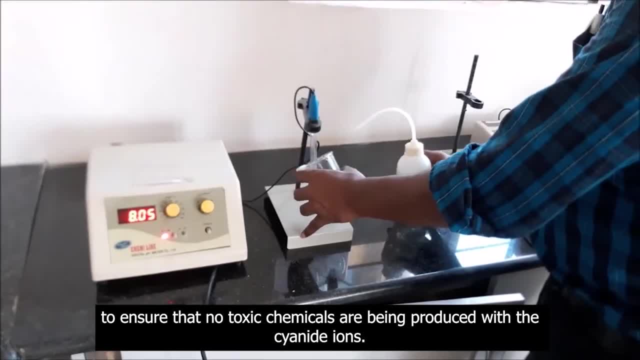 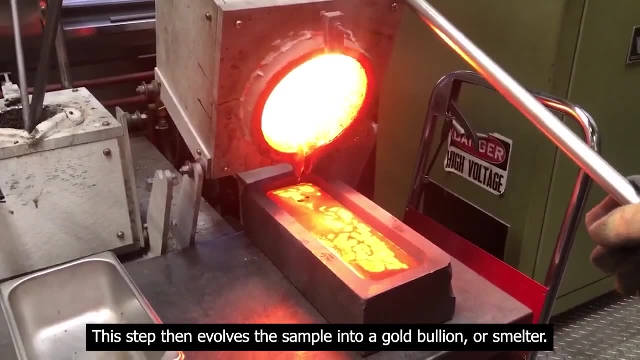 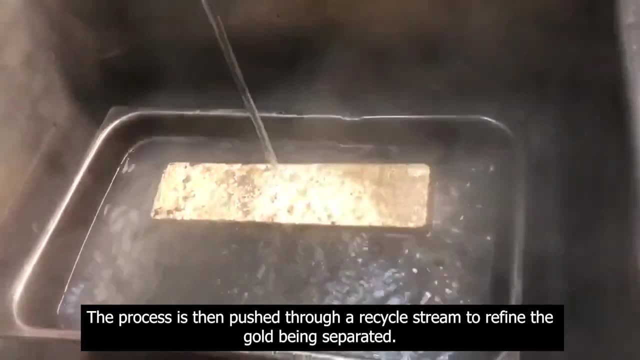 to ensure that no toxic chemicals are being produced with the cyanide ions. Third, concentrating and reducing the gold. This step then evolves the sample into a gold bullion or smelter. The process is then pushed through a recycle stream to refine, the gold being separated. 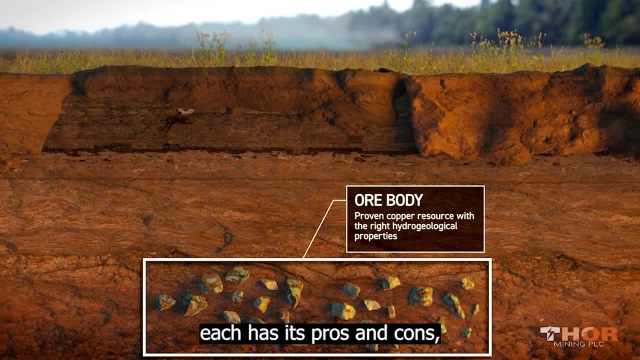 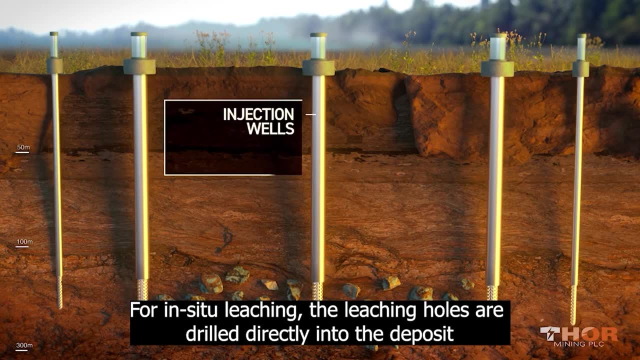 There are various types of leaching methods. Each has its pros and cons, And one of the most traditional leaching is called in-situ leaching. For in-situ leaching, the leaching holes are drilled directly into the deposit and the